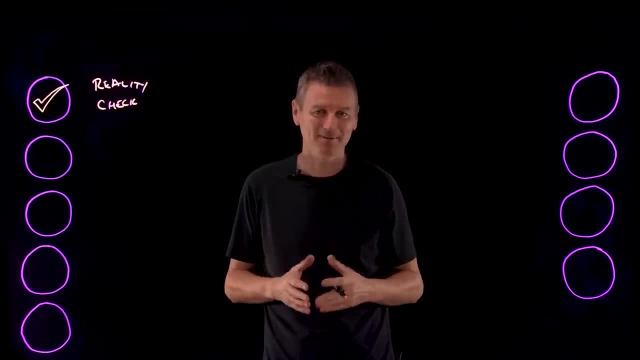 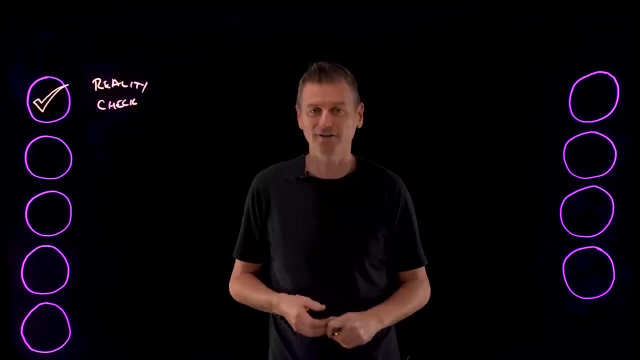 Now, many generative AI tools are now being implemented as integrated elements rather than standalone chatbots and the like. They enhance and complement existing tools rather than revolutionize or replace them. So think co-pilot features in Microsoft Office or generative fill in Adobe Photoshop, And embedding AI into everyday workflows like these helps us. 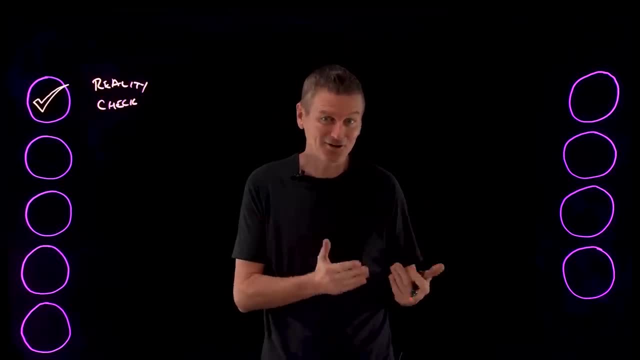 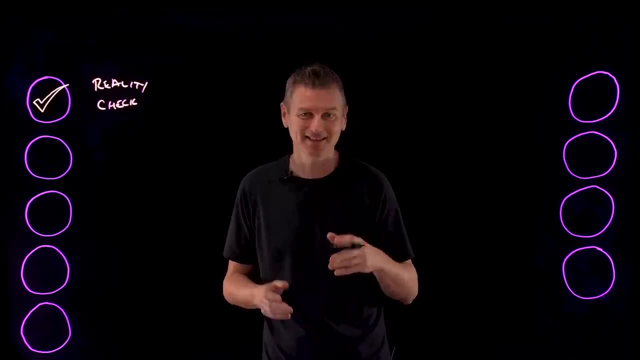 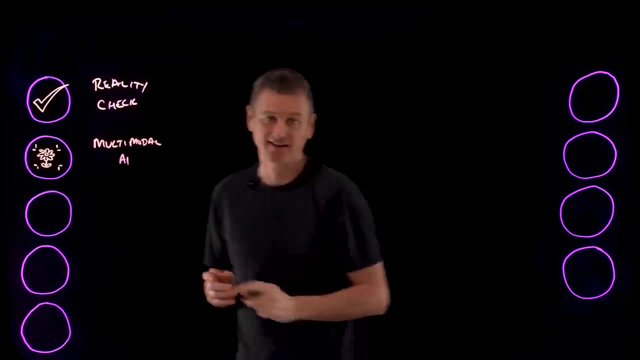 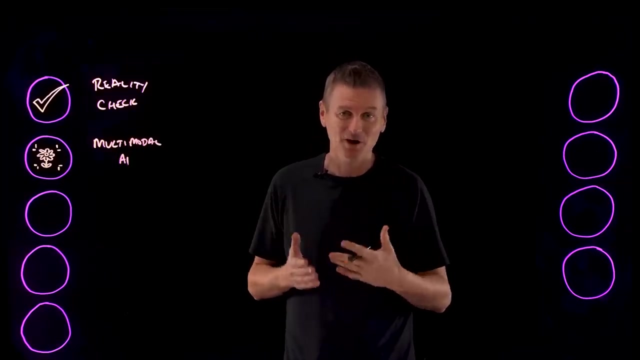 to better understand what generative AI can and cannot do in its current form, And one area generative AI is really extending its capabilities, That is in multi-modal AI. Now, AI multi-modal models can take multiple layers of data as input, And we already have 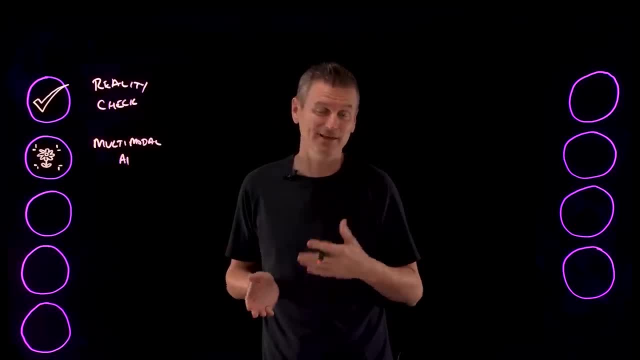 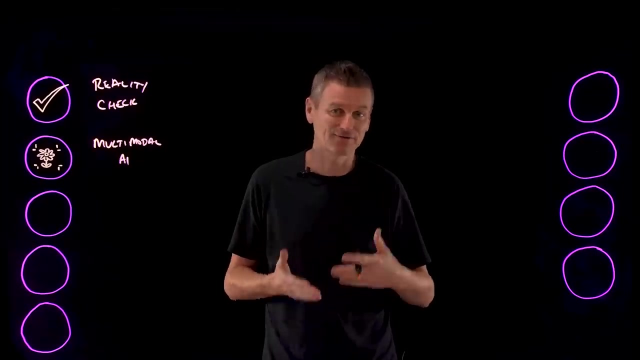 interdisciplinary models today, like OpenAI's GPT-4V and Google Gemini, that can move freely between natural language processing and computer vision tasks. So users can, for example, ask about an image and then receive a natural language answer, Or they could ask out loud for instructions to, let's say, repair something, and receive visual aids alongside. 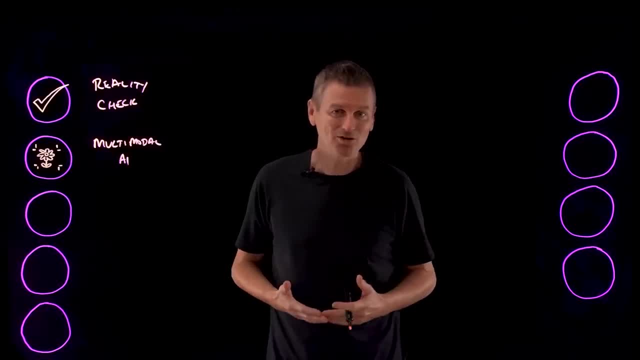 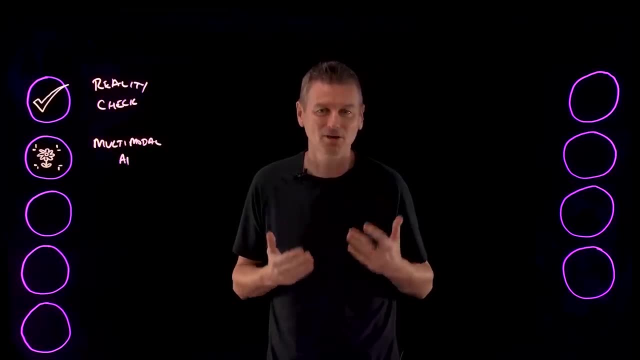 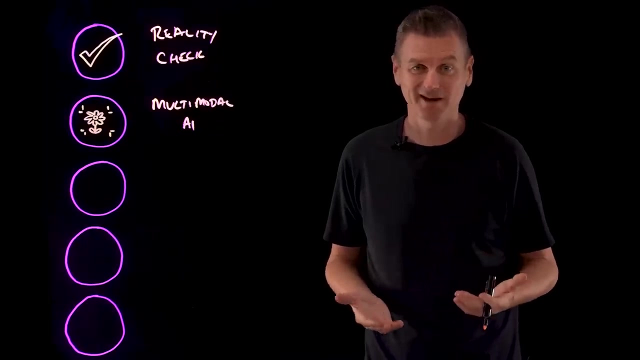 step-by-step text instructions. New models are also bringing video into the fold, And where this really gets interesting is in how multi-modal AI allows for models to process more diverse data inputs, And that expands the information available for training and inference, for example by 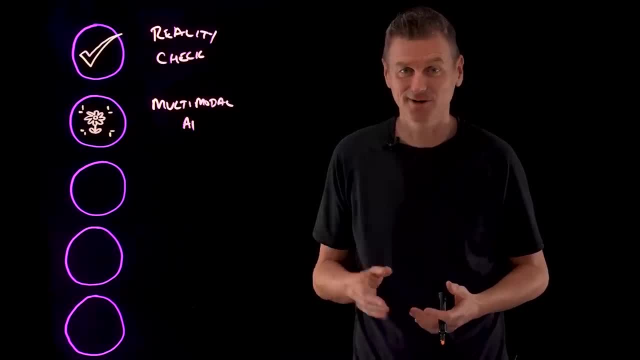 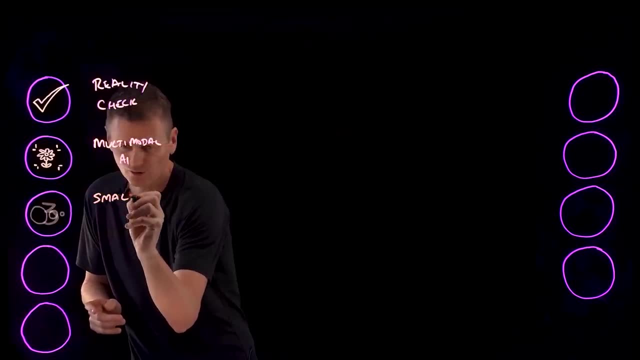 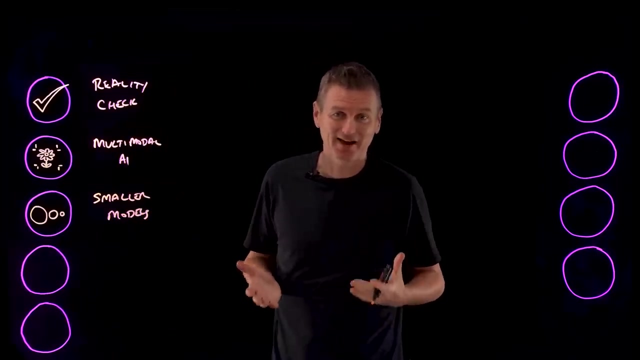 ingesting data captured by video cameras for holistic learning. So there's lots more to come this year. Now trend three. that relates to smaller models. Now massive models. they jumpstarted the generative AI age, but they're not without. 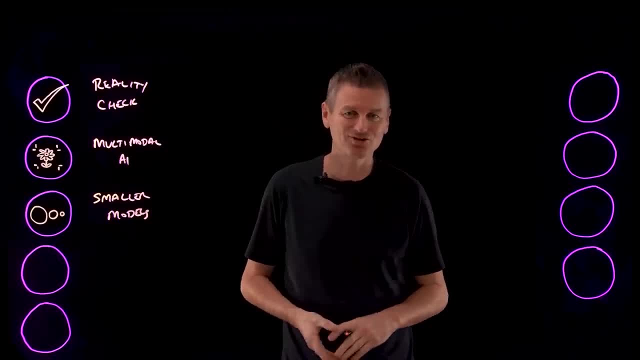 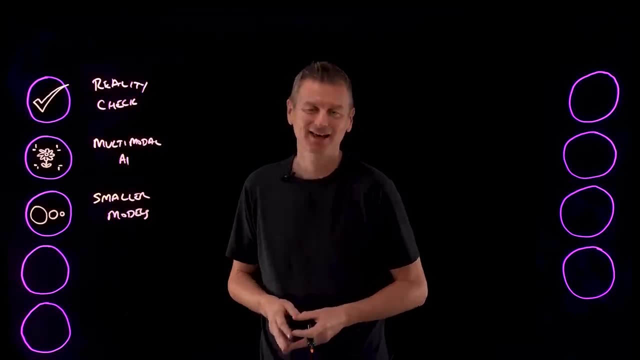 drawbacks. According to one estimate from the University of Washington, training a single GPT-3 size model requires the yearly electricity consumption of over a thousand households. And you might be thinking: sure, that's training, we know that's expensive. but what about inference? 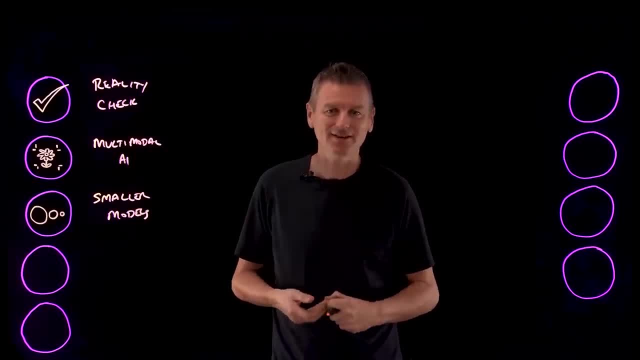 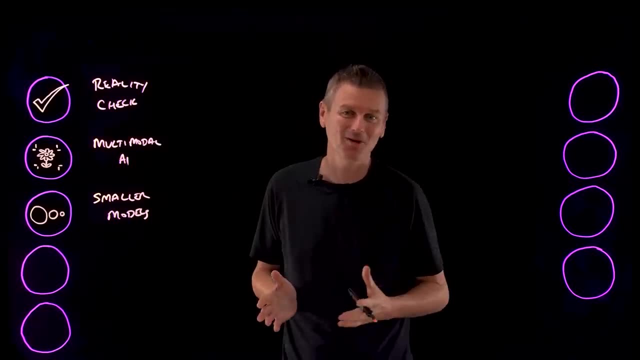 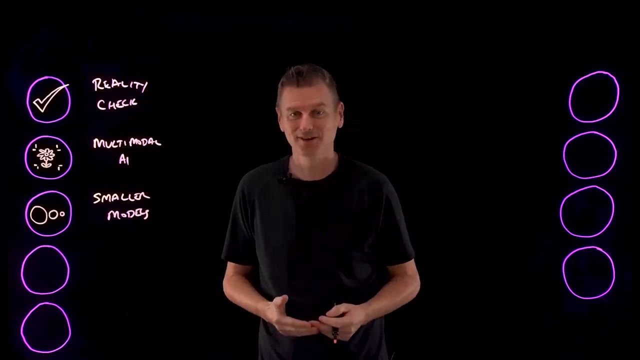 Well, a standard day of chat GPT queries rivals the daily energy consumption of something like 33,000 households. Smaller models, meanwhile, are far less resource-intensive. Much of the ongoing innovation in LLMs has focused on yielding greater output. 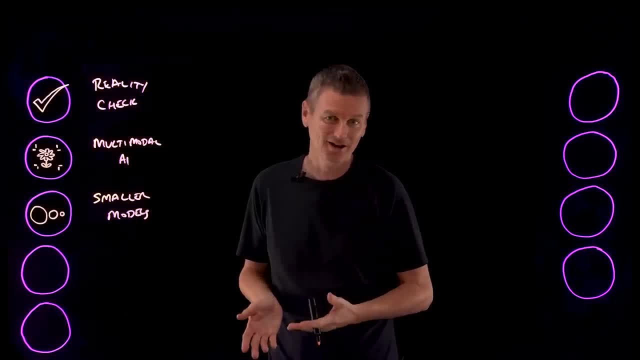 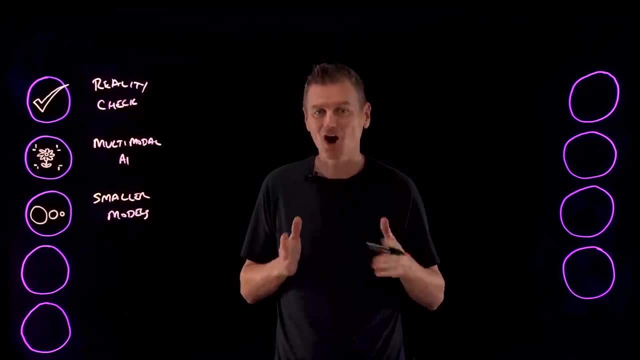 from fewer parameters. Now GPT-4, that is rumored to have around 1.7 billion cells per day in the body is a very high-dose, high-dose, high-dose model And the seven, six trillion parameters. but many open source models have seen success with model. 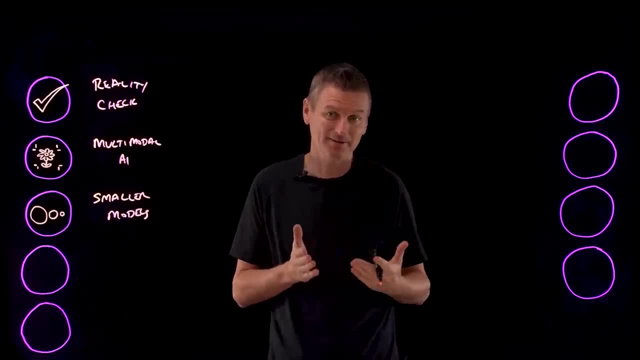 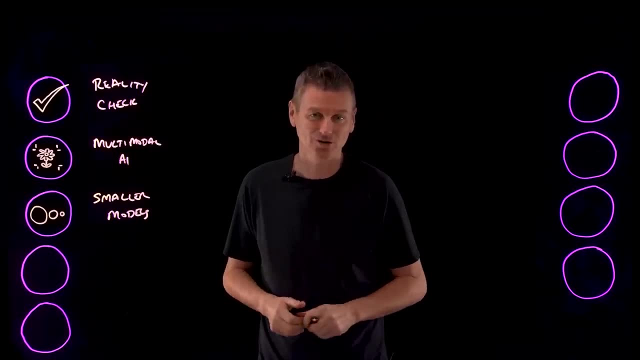 sizes in the three to 70 billion parameter range, So billions instead of trillions Now. in December last year, Mistral released Mixtral. That is a mixture of experts or an MOE model integrating eight neural networks, each with seven billion parameters, And Mistral claims. 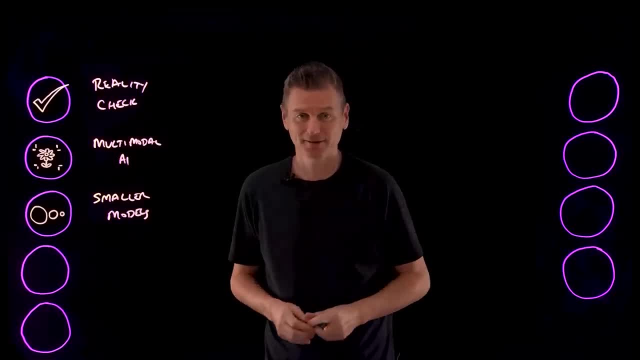 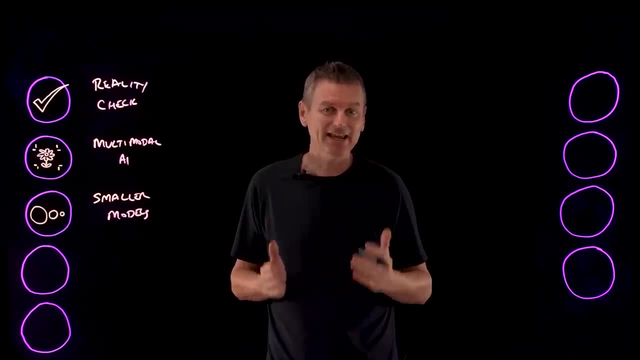 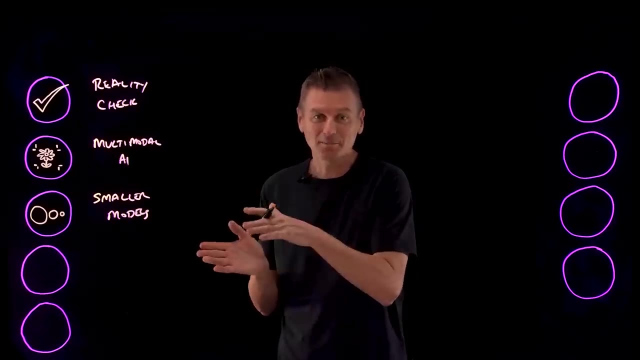 that Mixtral not only outperforms the 70 billion parameter variant of Lama 2 on most benchmarks at six times faster influence speeds, no less, but that it even matches or outperforms OpenAI's far larger GPT 3.5 on most standard benchmarks. Smaller parameter models can be run at lower cost. 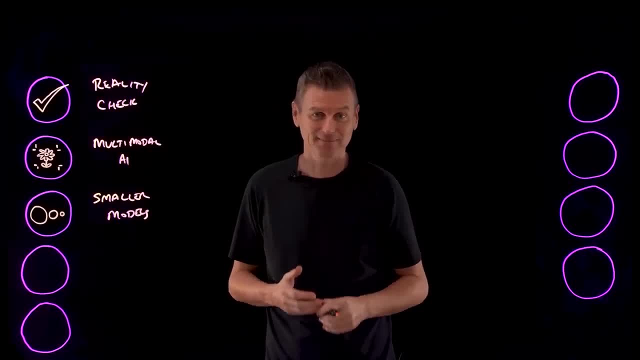 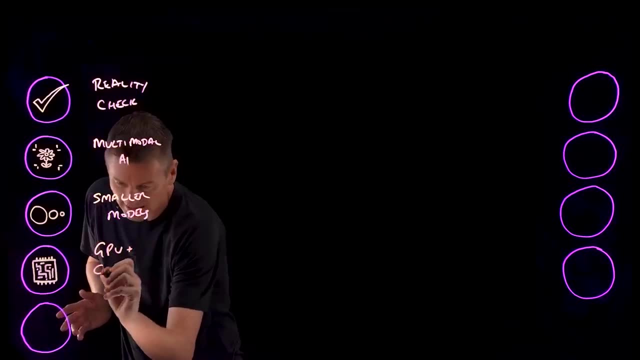 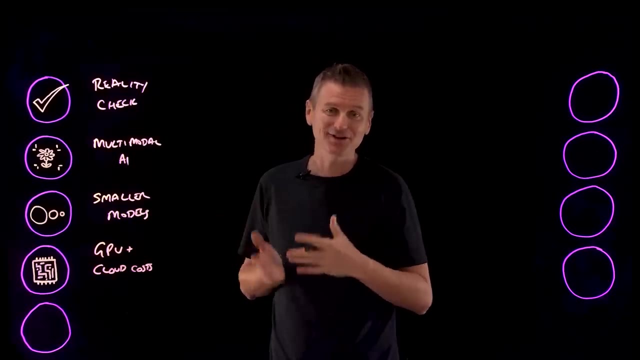 and run locally on many devices like personal laptops. Which, conversely, brings us to trend number four, which is GPU And cloud costs. The trend towards smaller models is being driven as much by necessity as it is by entrepreneurial vigor. The larger the model, the higher the requirement on GPUs. 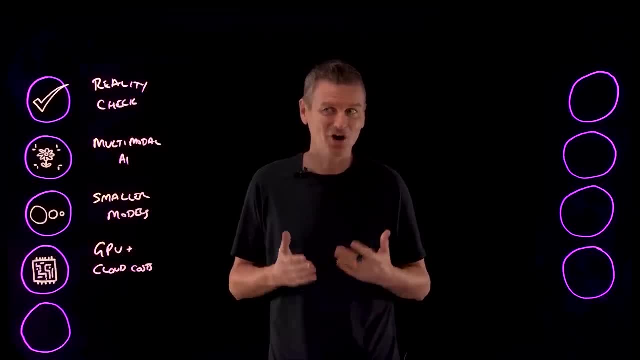 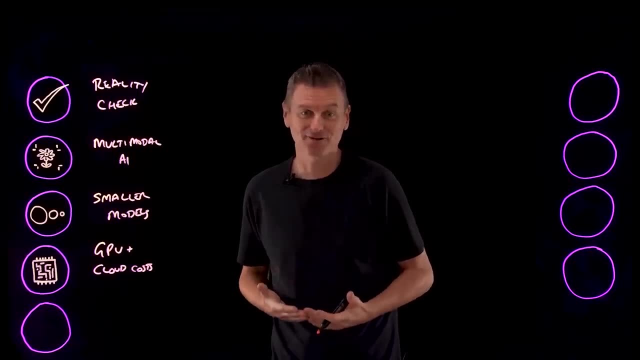 for training and inference. Relatively few AI adopters maintain their own infrastructure, So that puts upward pressure on cloud costs as providers update and optimize their own infrastructure to meet Gen AI demand, All while everybody is scrambling to obtain the necessary GPUs to power the infrastructure. 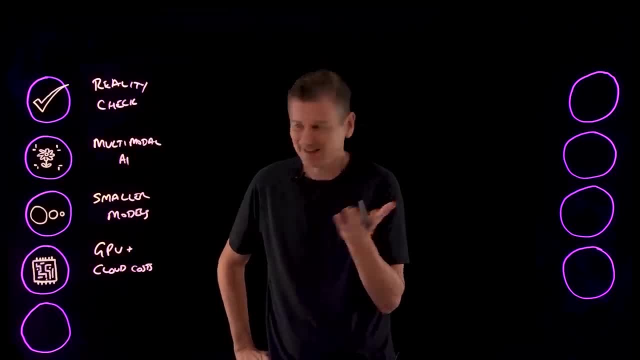 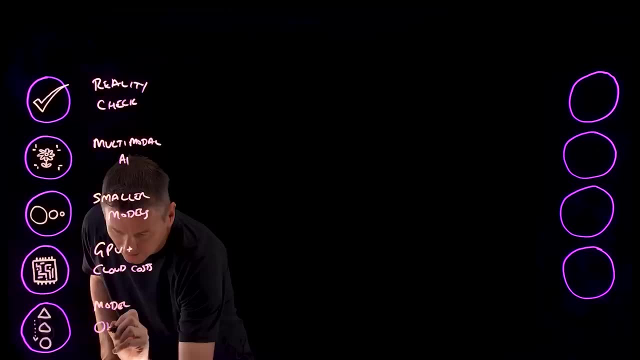 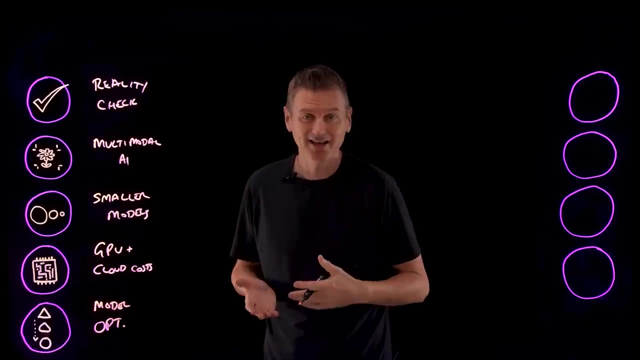 If only these models were a bit more optimized, they'd need less compute. Haha, yes, that is trend number five, That is model optimization. Now, this past year we've already seen adoption of techniques for training, tweaking and fine tuning pre-trained models, like quantization. You know how you can reduce the file size. 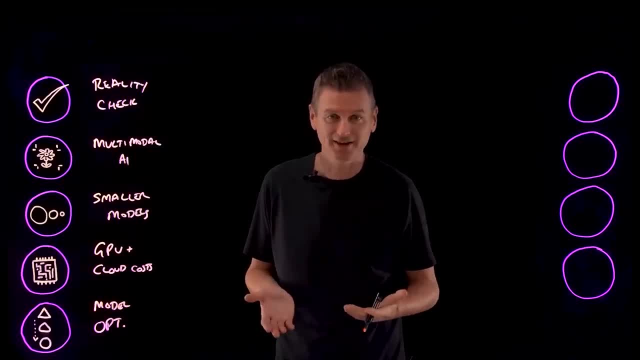 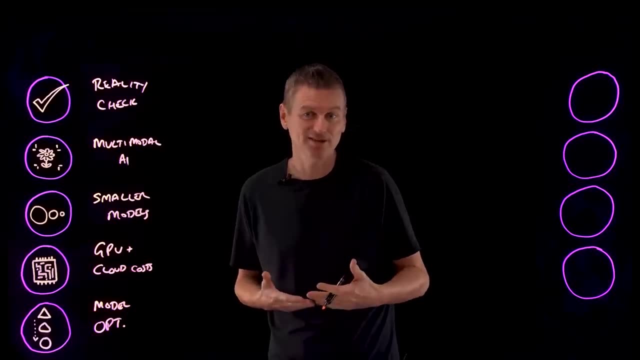 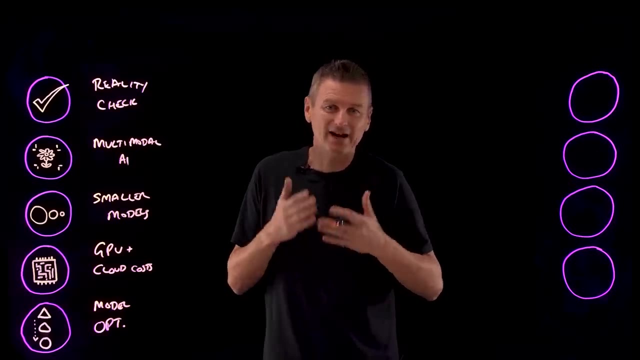 of an audio file just by lowering its bitrate. Well, quantization lowers the precision used to represent model data points, For example from 16 bit floating point to 8 bit integer, to reduce memory usage and speed up inference. Also, rather than directing directly, fine tuning billions of model parameters, something called 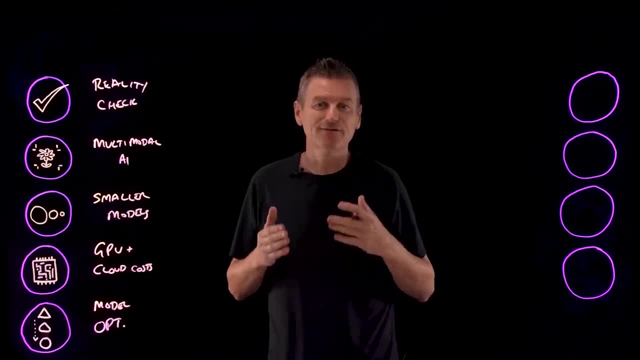 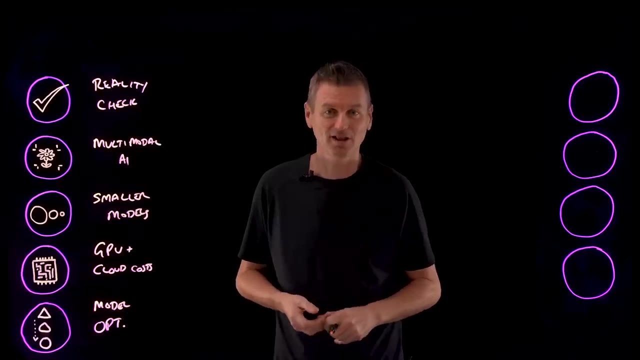 LoRa, or low rank adaptation, entails freezing pre-trained model weights and injecting trainable layers in each transformer block, And LoRa reduces the number of parameters that need to be updated, which in turn, dramatically speeds up fine tuning and reduces the memory needed to store model updates. 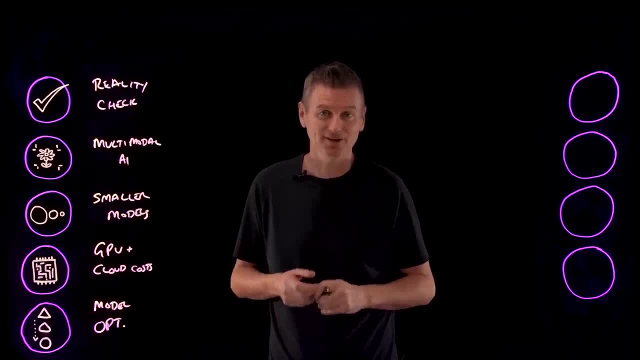 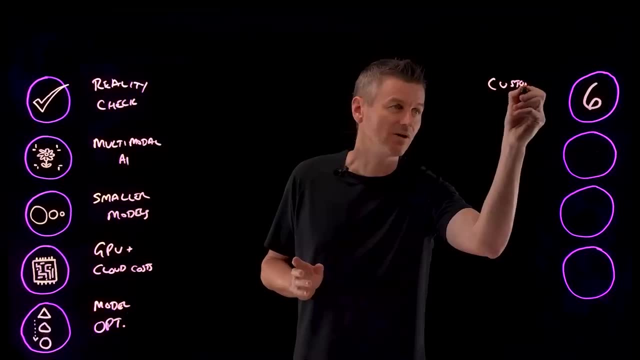 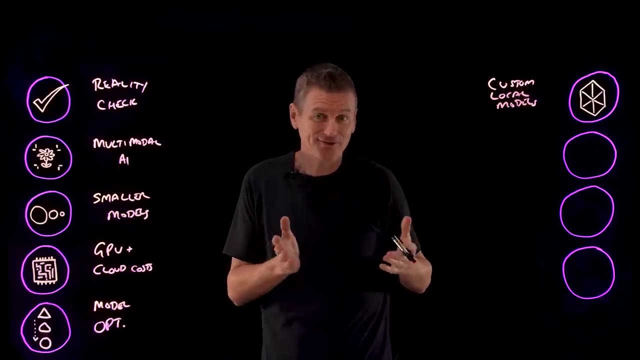 So expect to see more model optimization techniques emerge this year. OK, let's, let's knock out a few more, And the next one is all about custom local models. Open Source models afford the opportunity to develop powerful custom AI models. And when we talk about custom AI models, what are they? 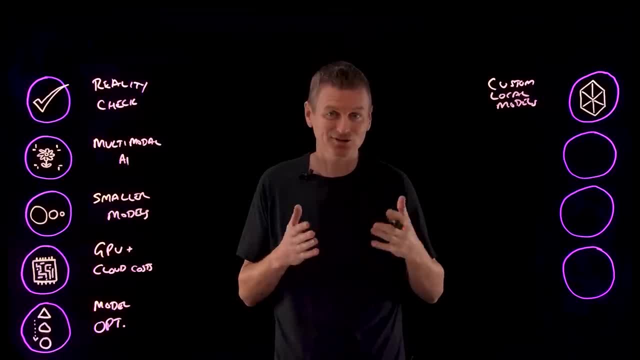 Well, open source models are a casual term. Open source models are often associated with software or software with the ability to use cloud-based models, or cloud-based models, or even cloud-based models. That means trained on an organization's proprietary data and fine-tuned for their specific needs. 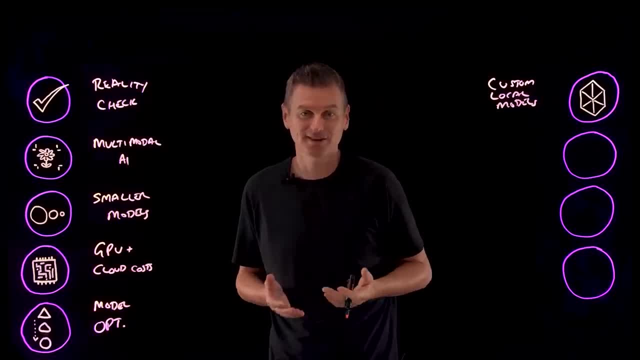 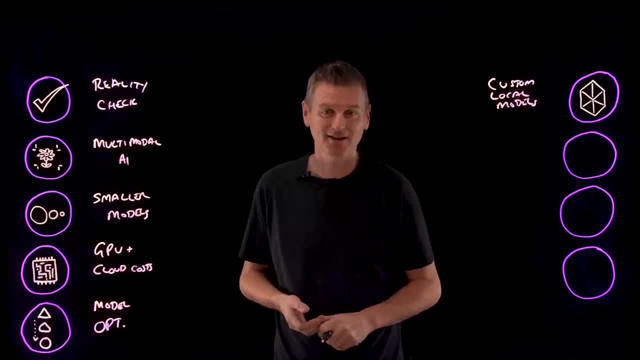 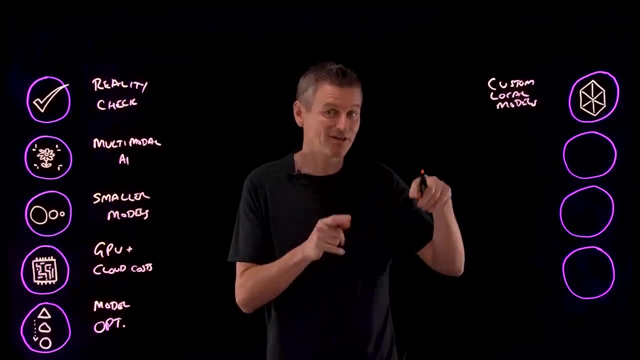 Keeping AI training and inference local avoids the risk of proprietary data or sensitive personal information being used to train closed source models or otherwise pass through to the hands of third parties And then using things like RAG or retrieval augmented generation to access relevant information, rather than storing all of that information directly within the LLM itself. that helps to reduce model size. 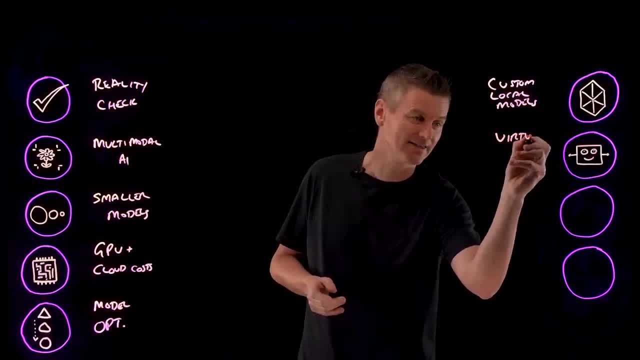 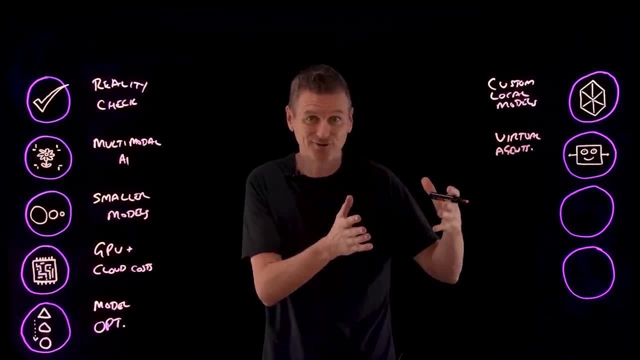 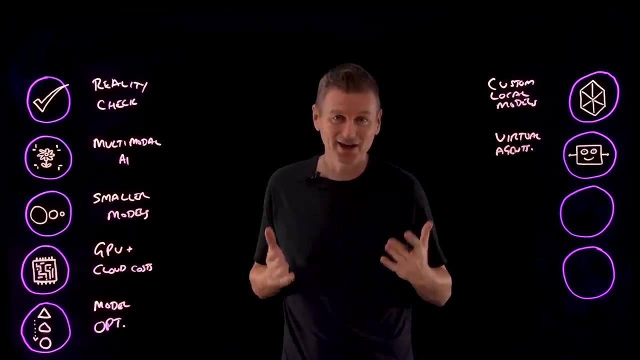 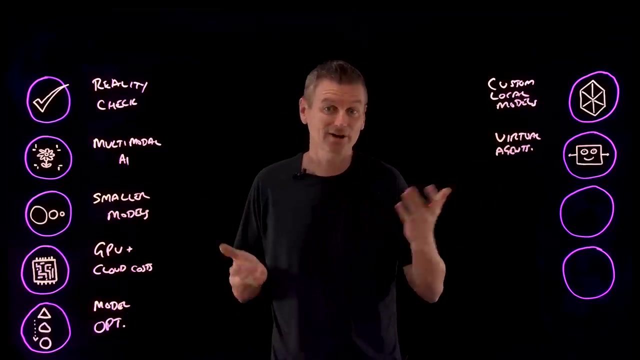 Trend number seven, that is, virtual agents. Now, that goes beyond the straightforward customer experience chatbot, because virtual agents relate to task automation, where agents will get stuff done for you: They'll make reservations or they'll complete checklist tasks or they'll connect to other services. 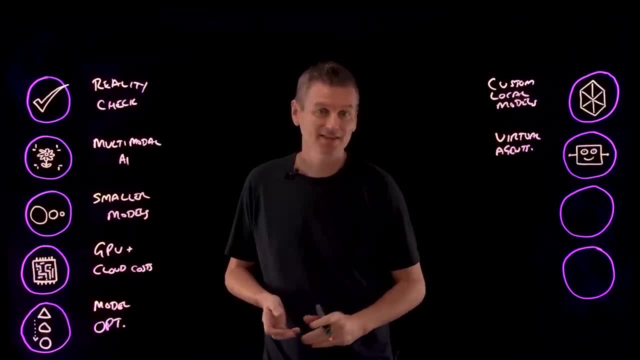 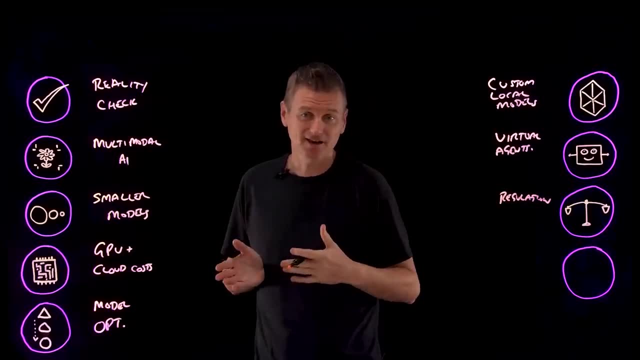 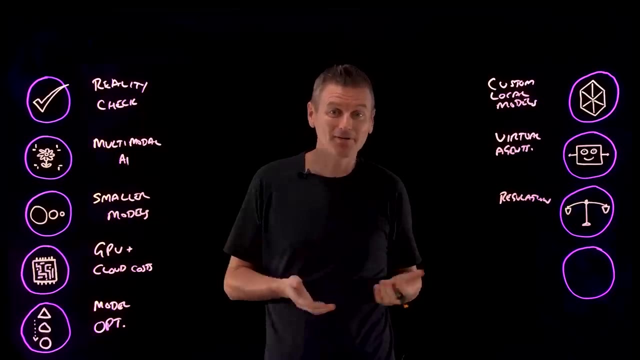 So lots more to come there. Trend number eight: That is all about regulation Now. in December of last year, the European Union reached provisional agreement on the Artificial Intelligence Act. Also, the role of copyrighted material in the training of AI models used for content generation remains a hotly contested issue. 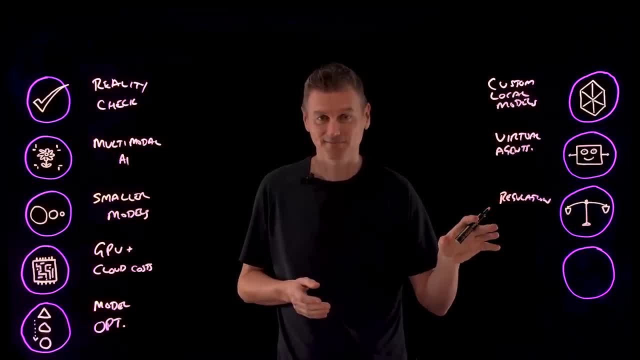 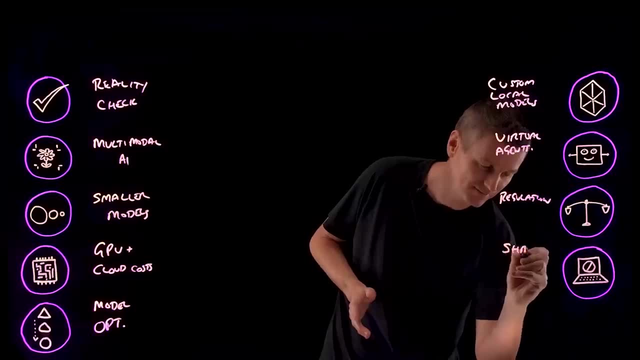 So expect much more to come in the area of regulation. And finally, we're at trend number nine, which is the continuance of something called AI. And finally, we're at trend number nine, which is the continuance of something called AI. 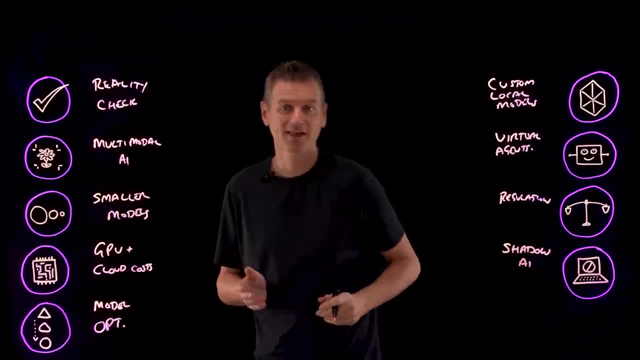 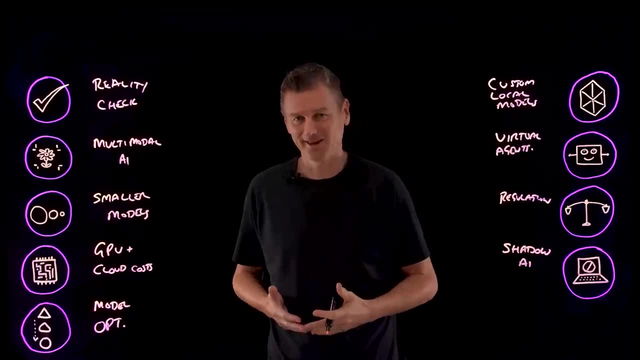 And finally, we're at trend number nine, which is the continuance of something called shadow AI. And finally, we're at trend number nine, which is the continuance of something called shadow AI. What's that? Well, it's the unofficial personal use of AI in the workplace by employees.